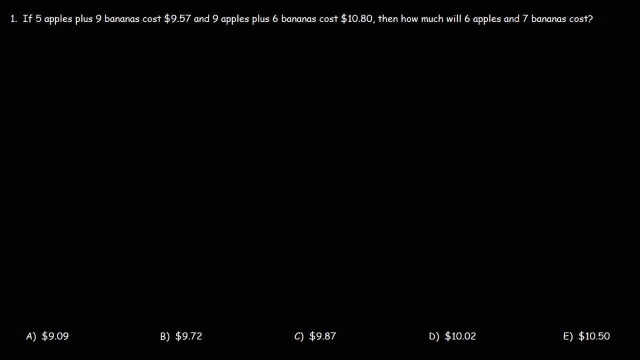 So feel free to pause the video and take a minute and try this problem, if you wish. Now the way to solve this is to write a list of equations. So the first part of the question helps us to write the first equation. So 5 apples- let's use A for apples- plus 9 bananas. 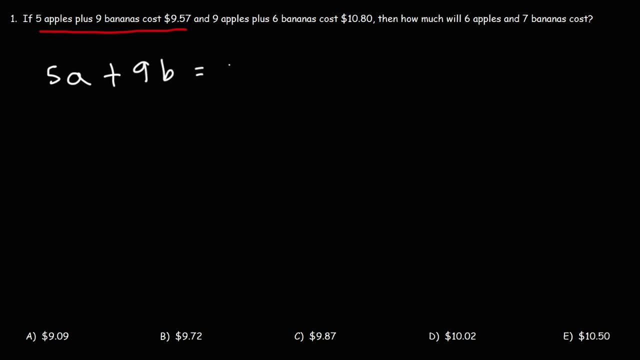 costs $9.57.. So we're going to say that's equal to 9.57.. That's the first equation that we have Now. we can also write another equation using the second part of the sentence, That is, 9 apples or 9A plus 6B. 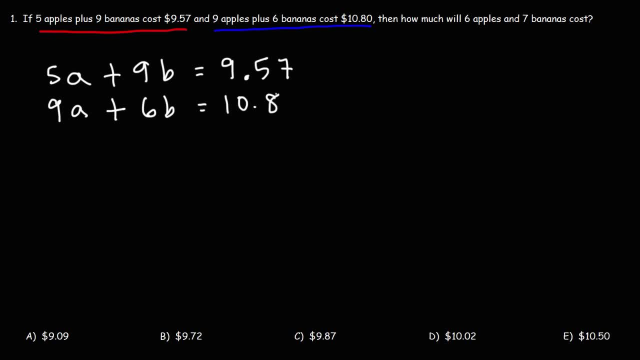 that's going to equal 10.80.. So what we have here is a system of linear equations. All we need is two equations to solve for two variables. Once we get the values of A and B, then we can answer the third part of the question. So how do we calculate the values of A and B? 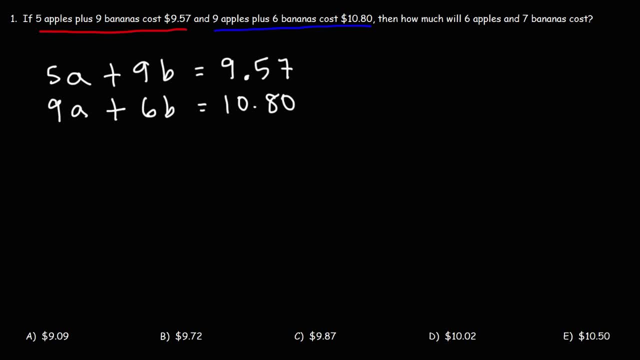 in this equation. We're going to use a process known as elimination. We're going to solve this system of equations by elimination, So we need to decide if we want to cancel A or B. Let's focus on B Now. what we can do is multiply. 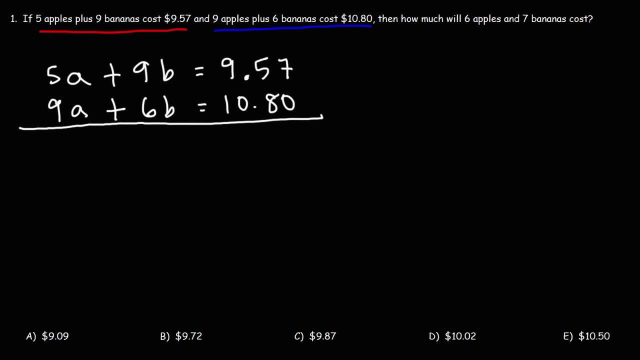 each equation by some number, such that when we add the two equations, the B variables will cancel. So we have 9 and 6.. What is the least common multiple of 9 and 6?? Multiples of 6 are 6,, 12,, 18,, 24, and so forth. 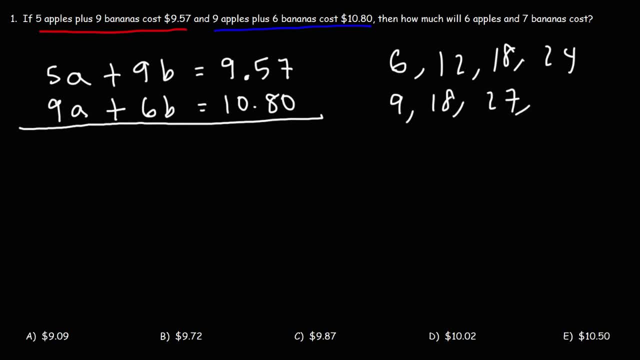 Multiples of 9 are 9,, 18, 27.. So 18 is the least common multiple of 9 and 6.. So what I'm going to do is I'm going to multiply the first equation by 2, because 18 divided by 9 is 2.. 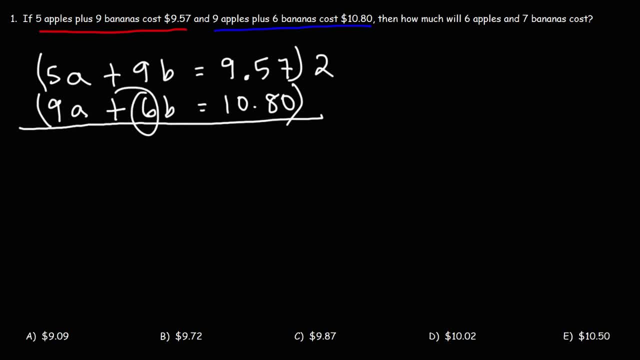 18 divided by 3, I mean by 6- is 3.. So I'm going to multiply the second equation by 3.. But rather by negative 3, because I want positive 18B in the first equation, negative 18B on the second equation, because those two numbers will add up to 0. 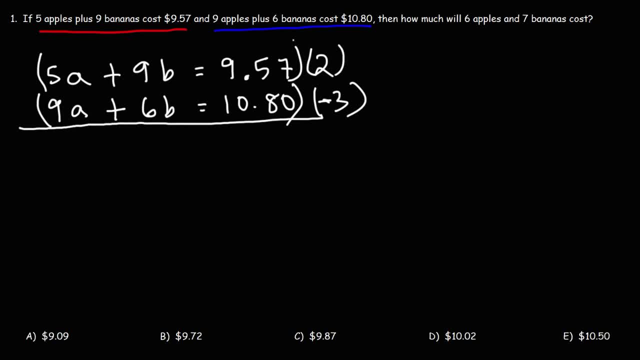 So let's multiply the first equation by 2.. So we have 5A times 2, which is 10A, 9B times 2, which is 18B, and then 9.57 times 2, which is 18B. 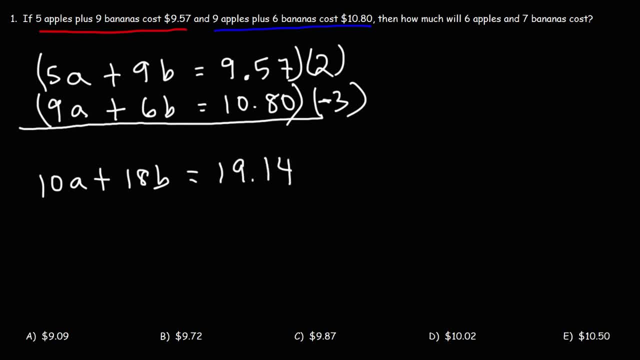 So that's going to be negative 18B. Now let's multiply the second equation by negative 3.. 9A times negative 3 is negative 27A. 6B times negative 3, that's going to be negative 18B. 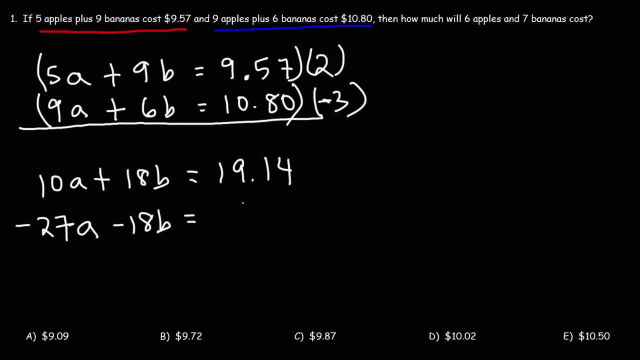 And then 10.8 times negative 3 is negative 32.40.. Now at this point we can add the two equations. Starting with the first column, we have positive 10 plus negative 27.. That's the same as 10 minus 27,. so that's going to give us negative 17,. and then times a. 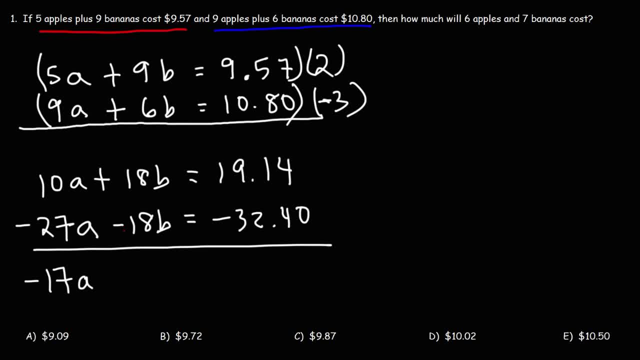 Positive 18b plus negative 18b. that adds up to 0, so they cancel. Thus this is called the elimination method, because we eliminated one of the variables from the two equations. Now add in the last two numbers 19.14 plus negative 32.40.. This is going to give us negative. 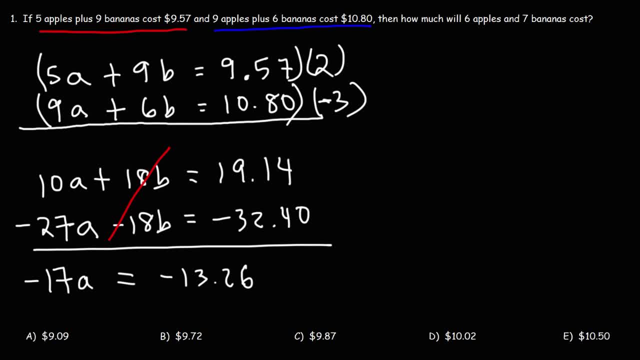 13.26.. Now to get a by itself, we need to divide both sides by negative 17.. So a is going to be negative 13.26 divided by negative 17.. So the cost of each apple is 78 cents. So now let's determine the cost of a single banana. 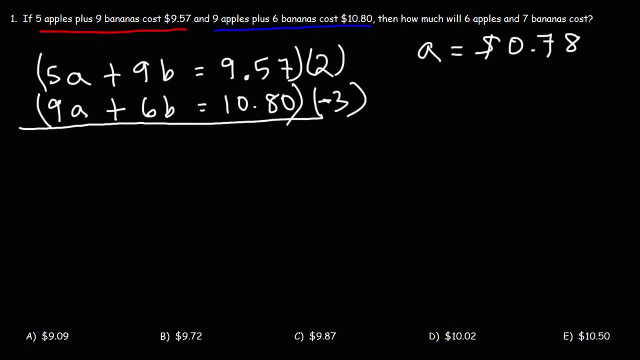 So let's use the first equation before we multiply it by two. So we're going to use this part of that equation. So let's replace a with 0.78, and let's calculate the value of b, So 5 times 0.78,, that's going to be 3.9, or you could say 3.90.. 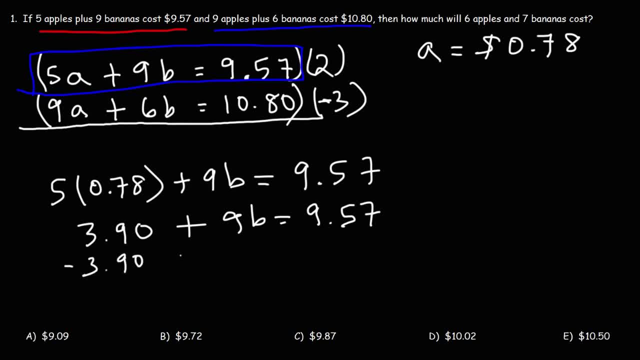 Now our next step is to subtract both sides by 3.9.. So we're going to get: 9b is equal to. now. let's subtract 9.57 by 3.9.. And this will give us 5.67.. Now the next thing we need to do is divide both sides by 9.. 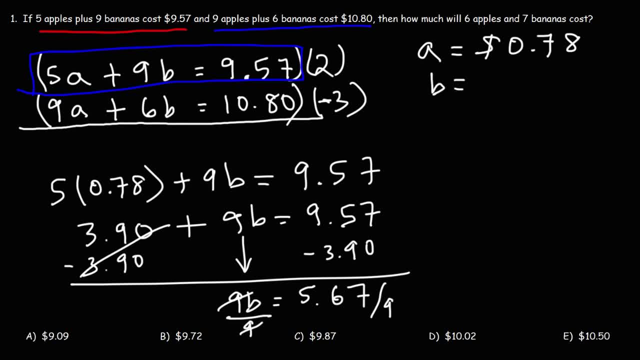 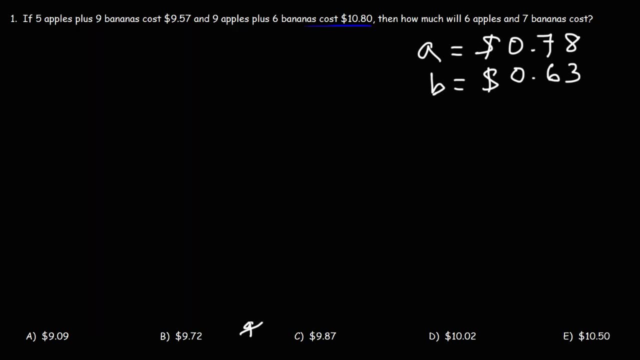 So b is going to equal 5.67 divided by 9, which is 0.63.. Therefore, the cost of each banana is 63 cents. So before we get the answer, let's make sure that the work we've done so far is correct. 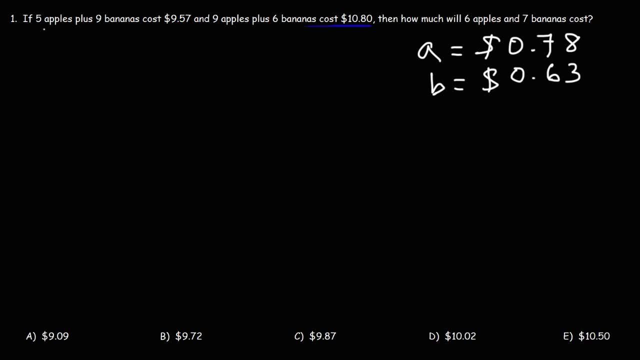 So let's make sure that 5 apples plus 9 bananas cost $9.57.. This will tell us that this information is correct. So 5 times 78 cents plus 9 times 63 cents, Is that equal to $9.57?. 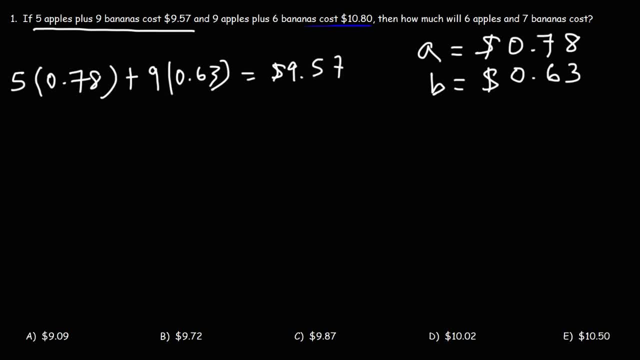 So 5 times 0.78, that's 3.9.. And 9 times 0.63 is 5.67.. So adding 3.9 and 5.67 gives us 9.57.. So those two values satisfies the first equation. Now let's make sure that it works for the second. 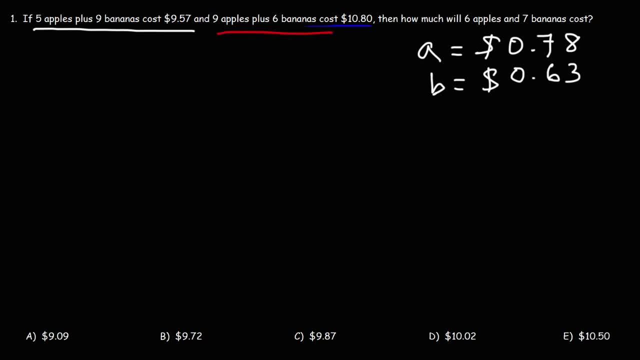 equation. So 9 apples, that's going to be 9.67.. 9 times 78 cents, plus 6 bananas, 6 times 63 cents, Let's see if that's equal to $10.80.. So 9 times 0.78,, that's 7.02.. 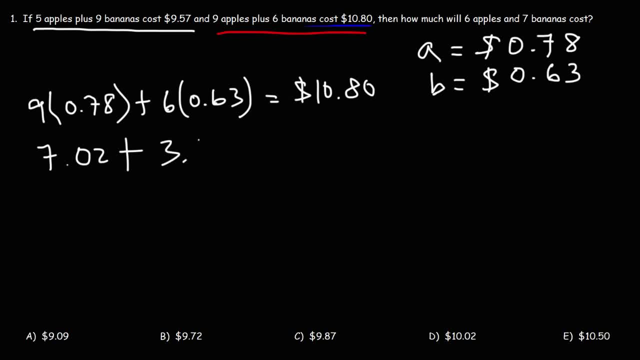 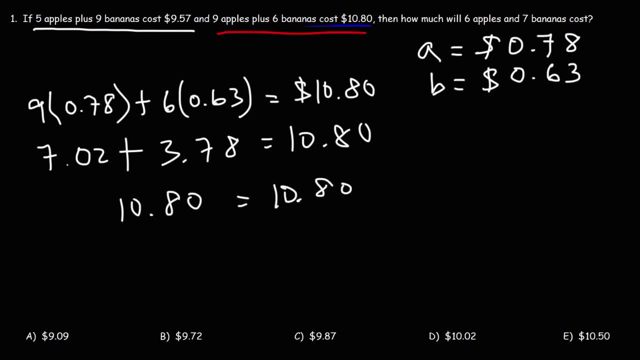 3.78 plus 7.02 is 10.02.. So both equations have been satisfied by these values, so we know that they're correct. So now that we have the cost of each individual apple and each individual banana, we can now